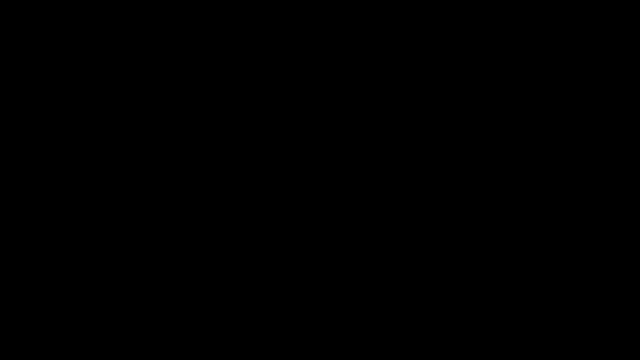 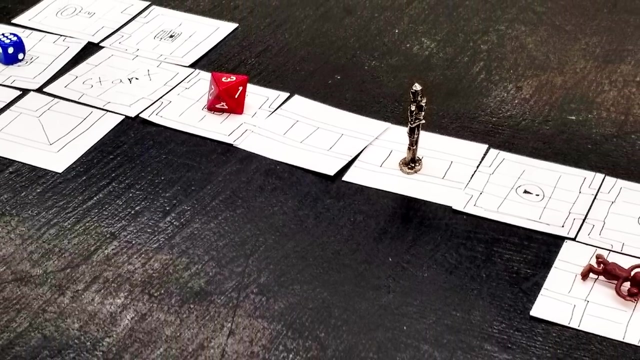 Today's episode is brought to you by Squarespace. Over three years ago, I created a roguelike board game while I was in college. At first it just was a fun project that I was doing for my friends, but then I was surprised to quickly see that people were interested in this game. That's. 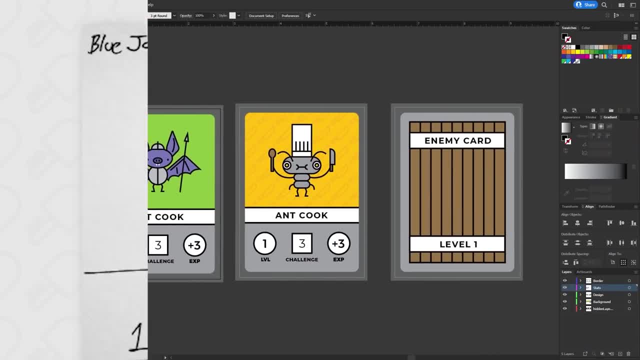 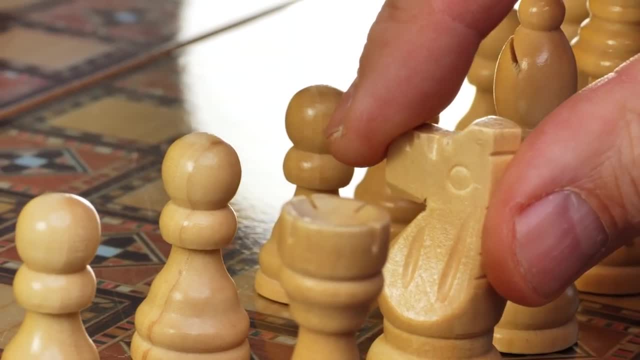 when I recruited one of my close friends, Brad, to help with the project. Now it took us a couple years to develop, but when we did release it we ended up selling a couple hundred copies. Unfortunately, like most things, the initial hype started to die out for the game. 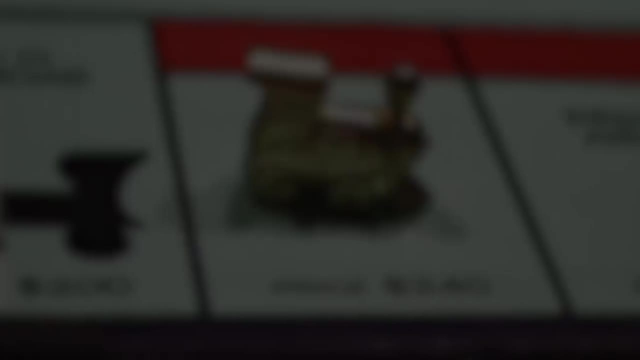 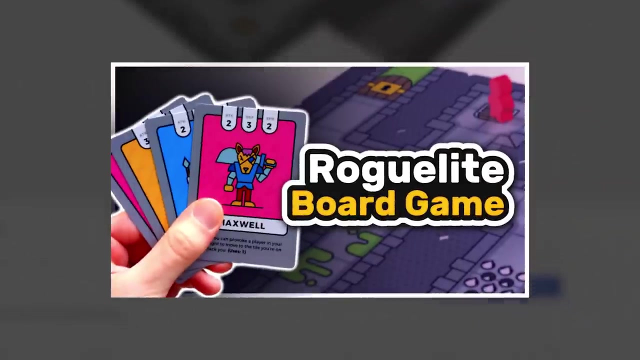 and eventually we kind of drifted away from the project. Now, if this story sounds a little bit familiar, that's because I'm talking about the Keep roguelike board game and I did a whole video on it earlier this year. And if that's the case, why am I doing another video on it now? 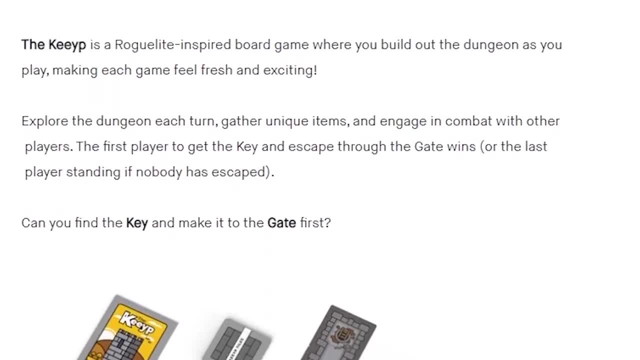 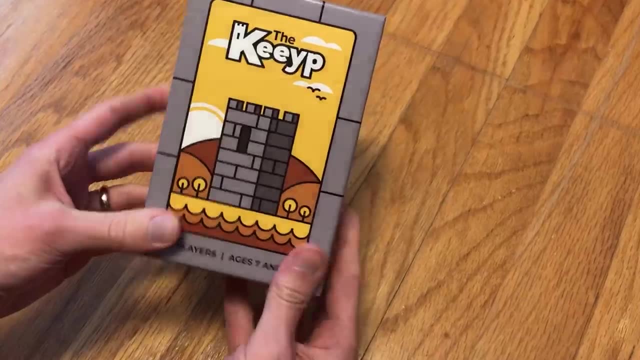 Well, I wanted to talk about everything that's happened since that video- and, believe me, there's a lot- And I also want to talk about the future of the Keep, for those who are still interested. So, without further ado, let's get started. 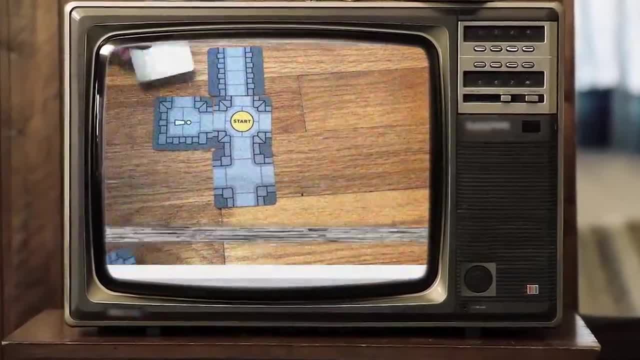 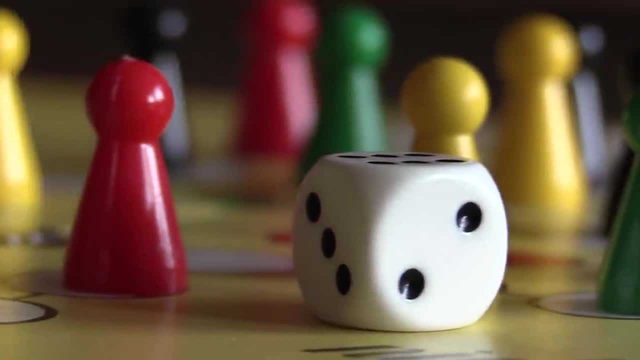 I mentioned that I created a video talking about the Keep and its story. Now the funny thing about that video is that was supposed to be kind of the farewell to the game. At that point no one was really buying copies or interested in it. So I thought, hey, I'm going to tell the story because 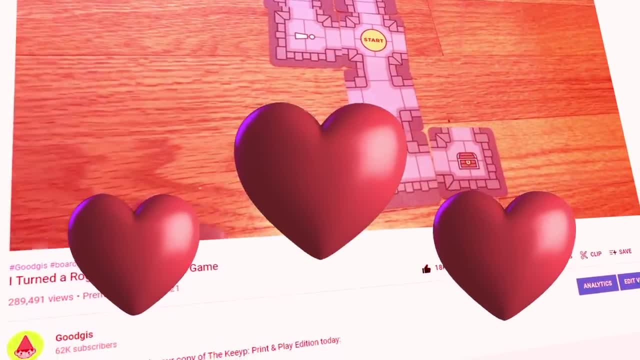 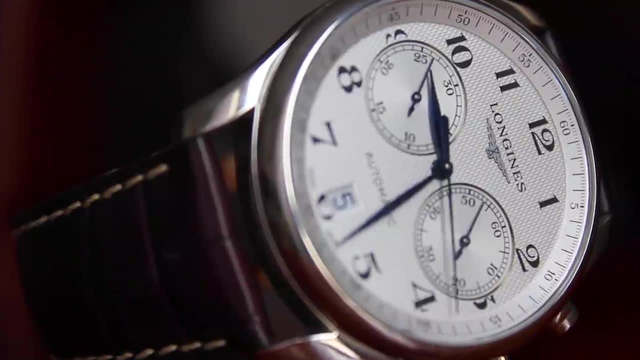 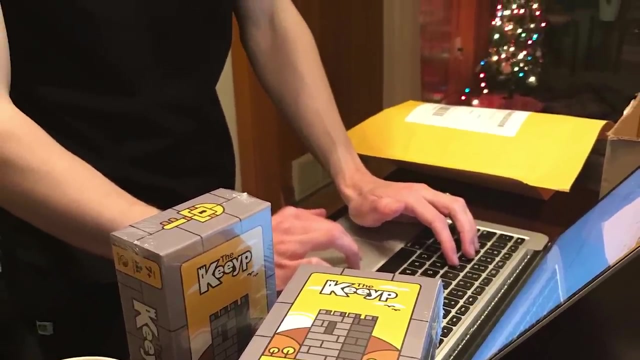 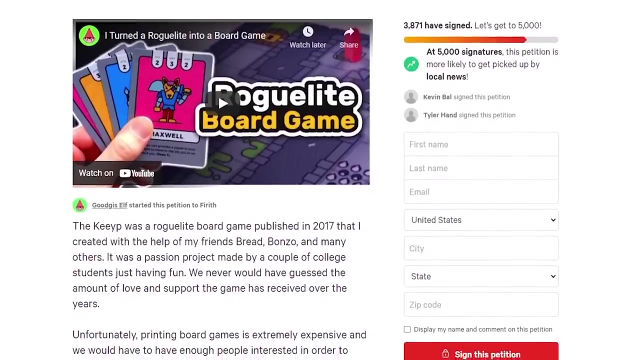 I'm proud of this game and we'll put it out there. If people want to buy the copies, that's fine, But after that the Keep is dead Boy. was I wrong? So I made a petition. My thought is that would be a way that we could find how many people were. 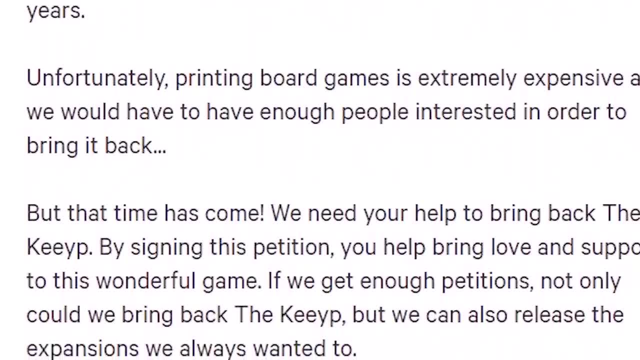 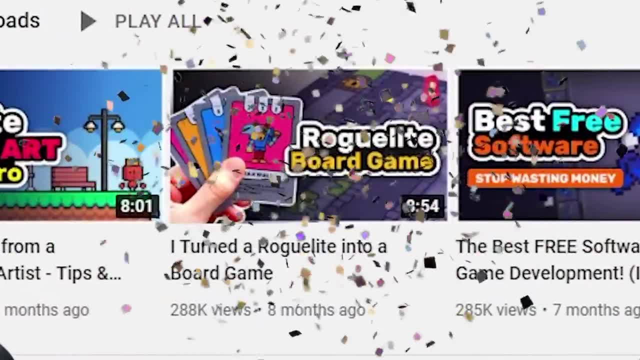 interested in buying the game so we could do a Kickstarter in a week or two. And I don't know if it was the petition or just the video itself, but the video blew up and is one of my most popular videos on this channel, And that's when I knew that I was going to do a Kickstarter And I was 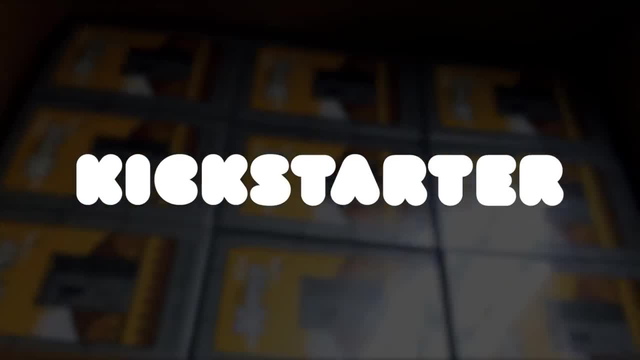 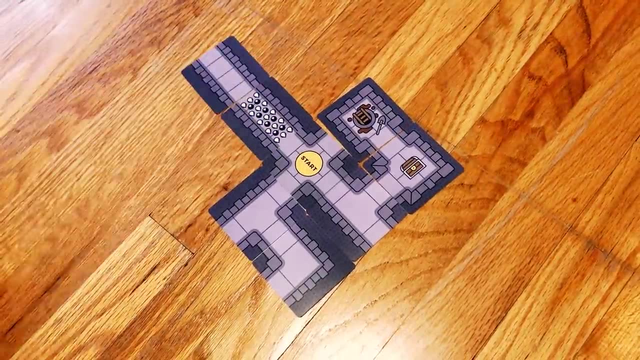 we needed to revive the keep, and this time we put it on kickstarter. now, if you don't know what the keep is, for some reason it's a roguelike board game where you actually have to build out the map each turn. your goal is to search and find a key. before you find the key, everyone's friendly and 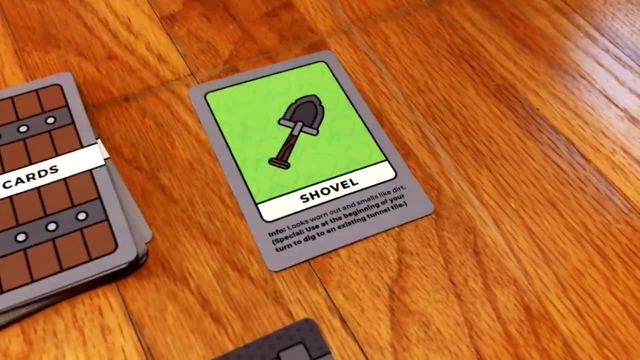 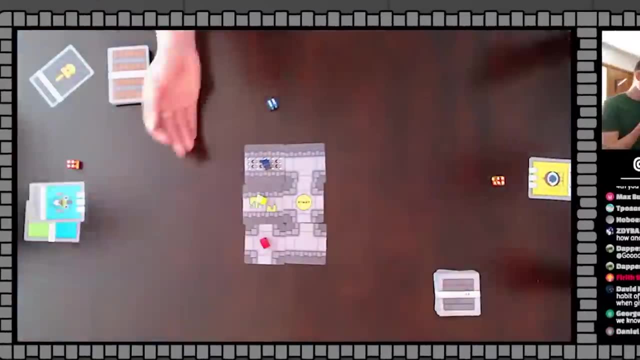 you have a fun time collecting items, but after the key, everyone turns on each other and your goal is to do one thing, and that's to get to the gate as fast as humanly possible. and one thing i love about it is that no two games are quite the same okay. so now that you know a little bit about 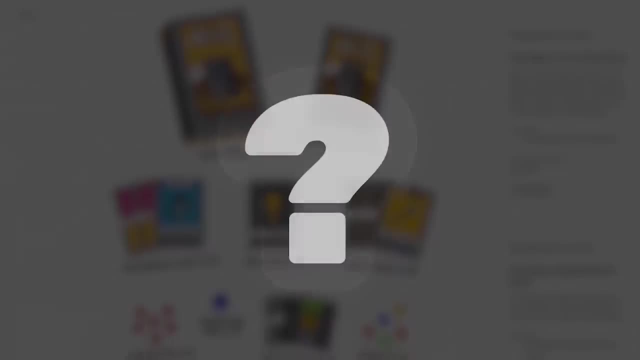 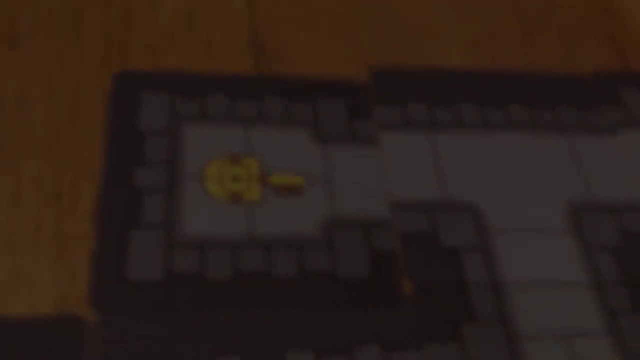 the game and the setting up for the kickstarter. you're probably wondering how it all turned out in the end. so once we finally released the kickstarter, we were funded within 24 hours. not only that, but we ended up raising a total of thirty six thousand dollars, which is phenomenal. 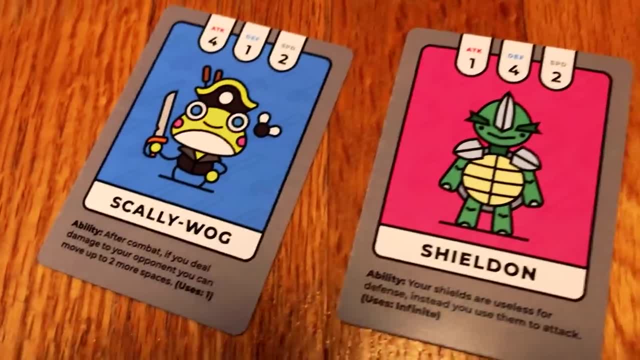 it allowed us to add custom dice and new keep links to the game, which really adds so much. okay, so we had a successful kickstarter, but that would make for a boring video if we were going to make a video about the game. so we're going to make a video about the game. 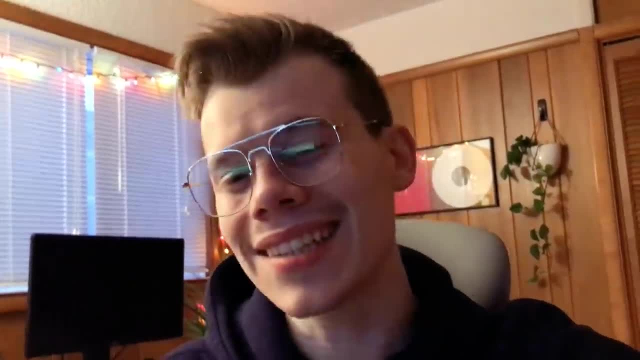 so we had a successful kickstarter, but that would make for a boring video if we were going to make only talked about that. so i wanted to share one of the mistakes that i made during this kickstarter so maybe you can avoid it if you do one in the future. but before we do that, 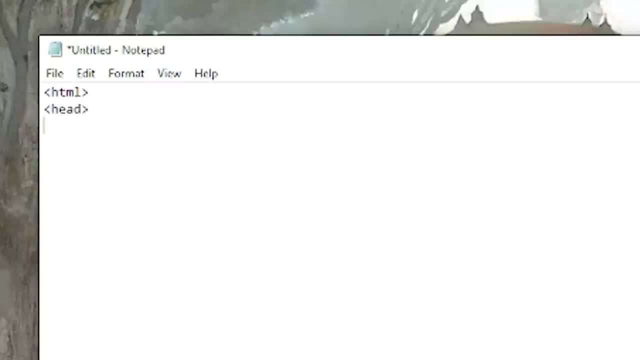 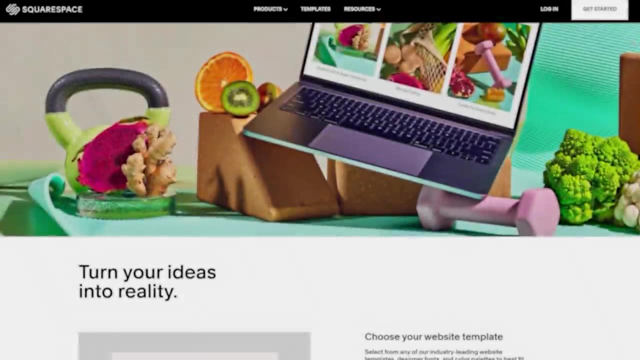 a word from today's sponsor, squarespace. making your own website or online store can be a huge pain in the butt from scratch. believe me, i've done it many times before, and the best way to cut the hassle is to use squarespace from selling your products online. 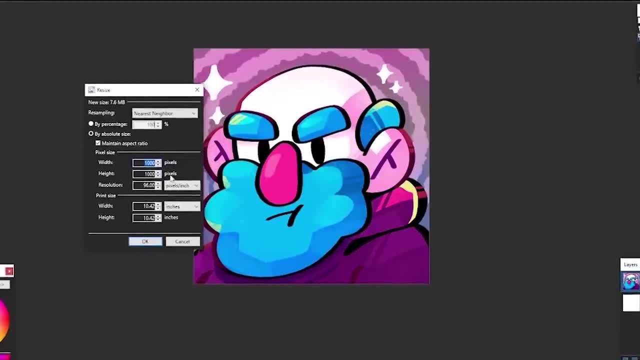 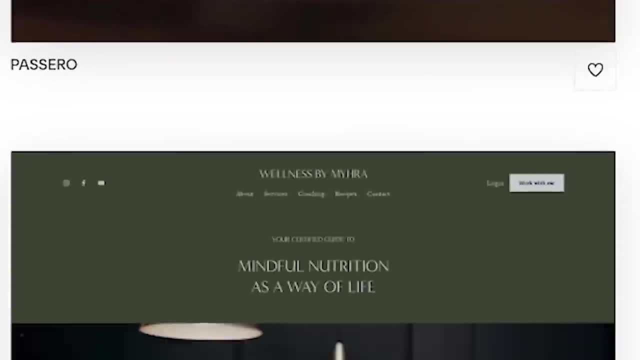 making a portfolio or gallery of your work, or even something as tedious as image scaling, is so much easier and saves you so much time. with squarespace, as the internet expands, i truly believe that everyone should have internet real estate, but creating your own website doesn't mean you have. 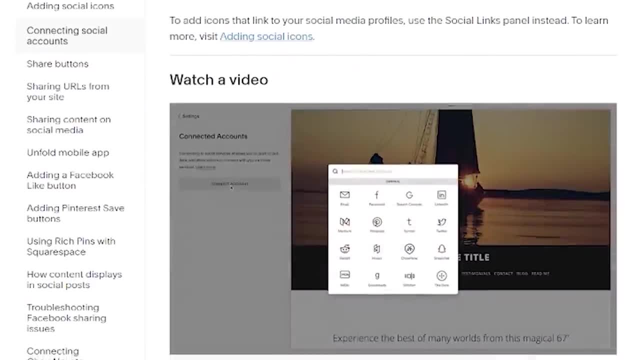 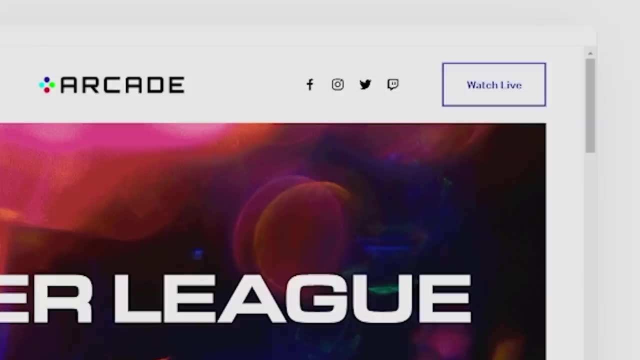 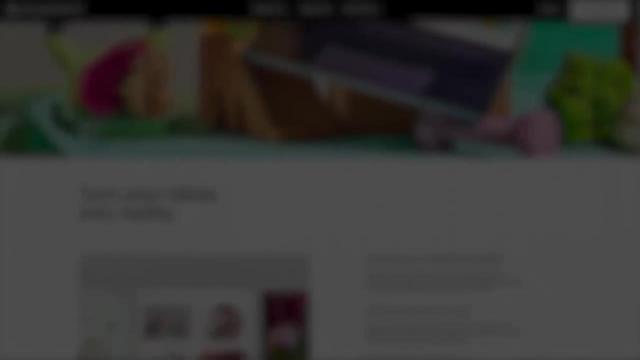 to be disconnected from social media. with squarespace, you can connect your social profiles so that way you can instantly post on different platforms, making it fantastic and easy to post your new product or game. make sure to go check out squarespacecom for a free trial and when you're ready, you're all set to launch. go to squarespacecom. good guess to save 10 percent on. 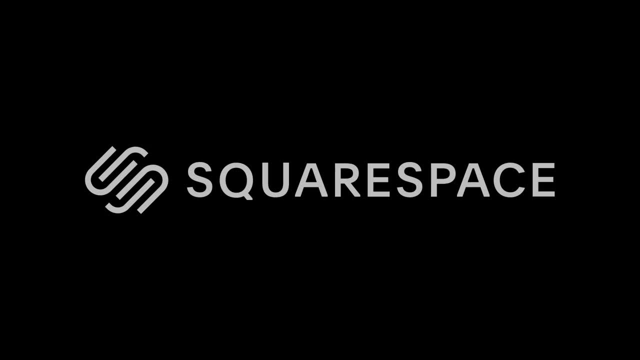 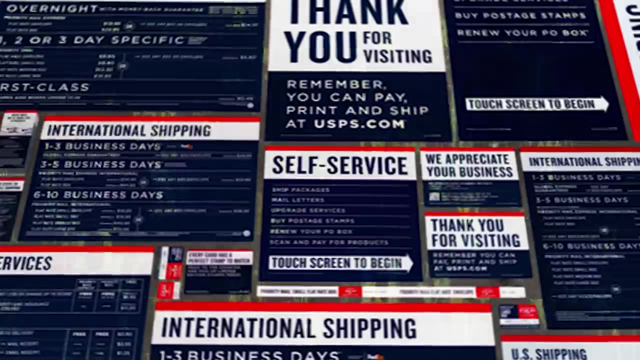 off your first purchase of a website or domain. one of the biggest issues we had during all of this was trying to figure out fulfillment. if you've ever done shipping before, it could be a huge pain in the butt. so when we first thought about doing this, we thought, hey, let's have our printers. 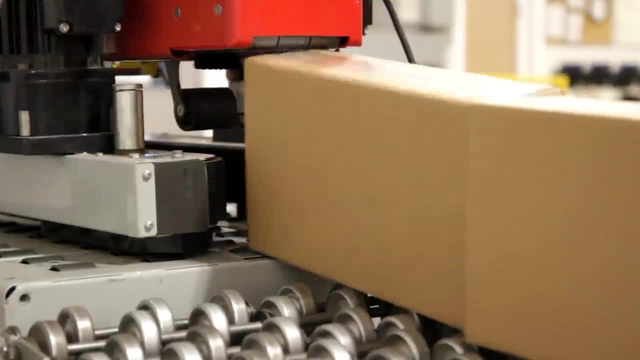 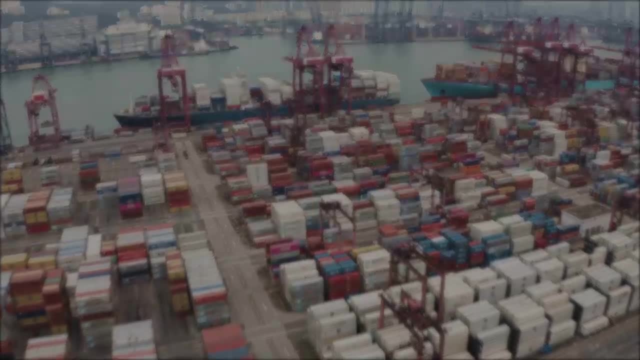 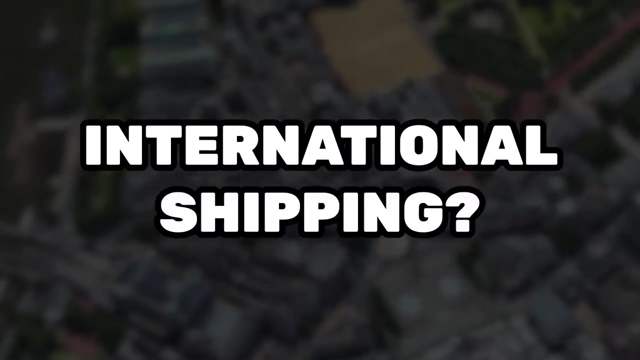 actually do all the fulfillment for us, so we can just do the kickstarter and not have to do all the grunt work. let's all find a danny for people in the us, but when it came to shipping stuff out of the way, we realized that a lot of people were not willing to pay $100 for shipping per game, which 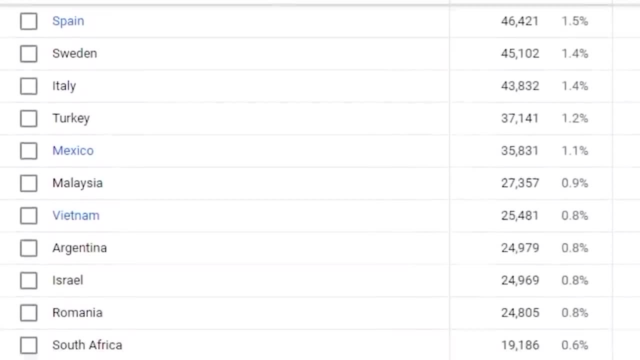 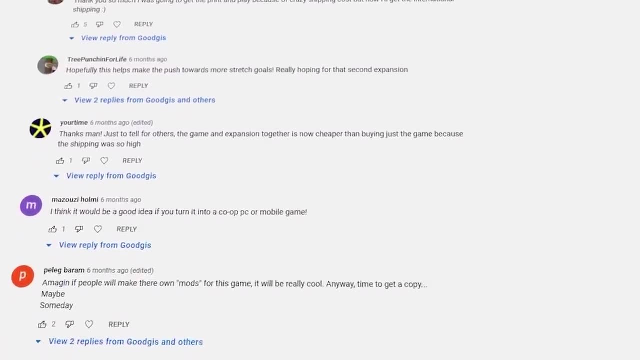 is insane. so we thought: how about we only make this in the us? well, that also was a huge mistake too, because there's a lot of people overseas that watch these videos and that would want a copy. so we quickly got a lot of comments of people saying, hey, at least give us the option. so sure enough. 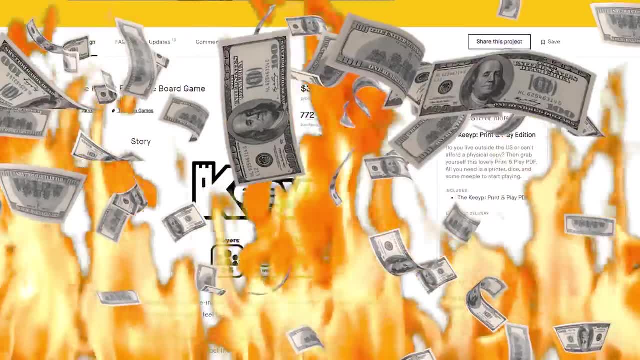 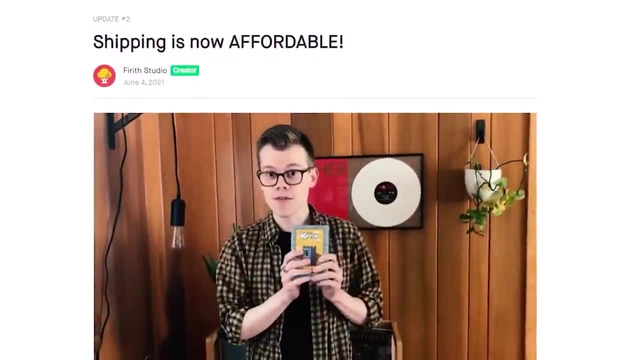 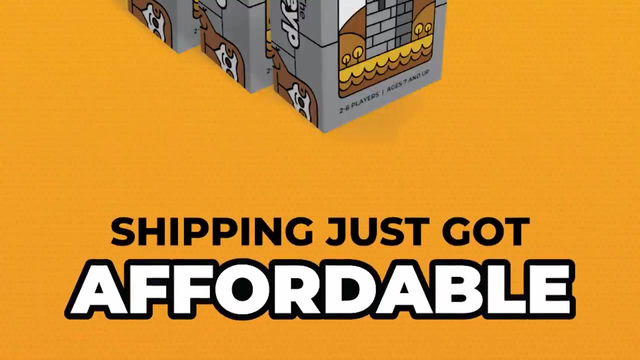 when the kickstarter launched, we had a ton of complaints from people that were just so mad about the price- and, like i said, i don't blame you whatsoever. so instead we found out that if we shipped out the copies ourselves, we could cut the price tag in half, which in my mind was a lot better, but it also meant a ton of work for us. one of the 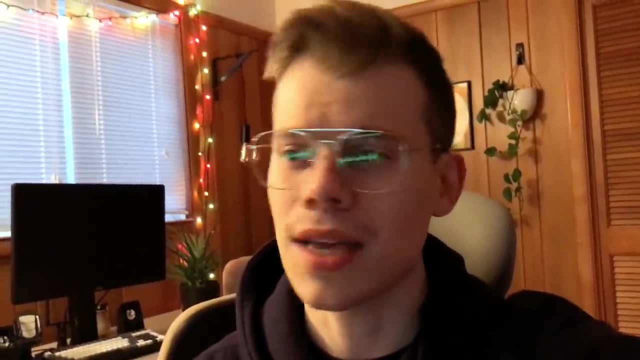 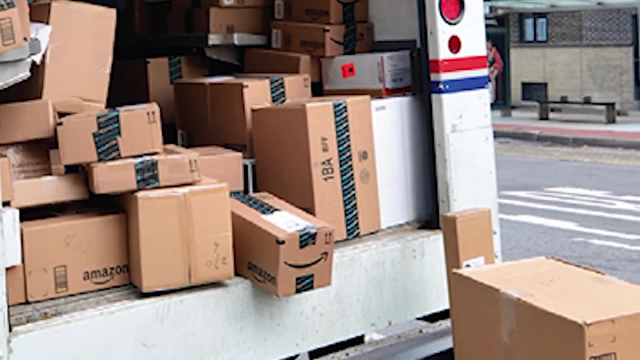 most important things for me is that you guys can play and enjoy the games, and that means, if i have to do some extra work in order for you guys to play it, then that's what i'm going to do. let's ship out some games. so, instead of the printers shipping out the copies, we actually got the mail. 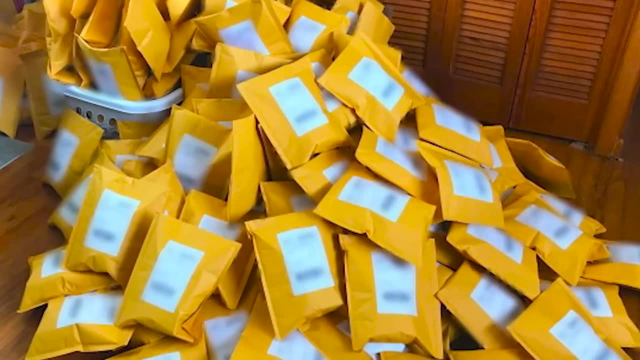 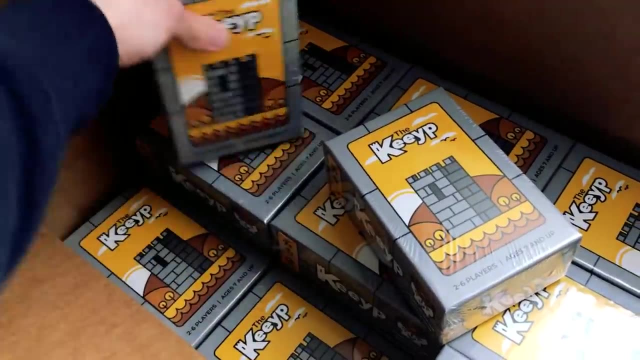 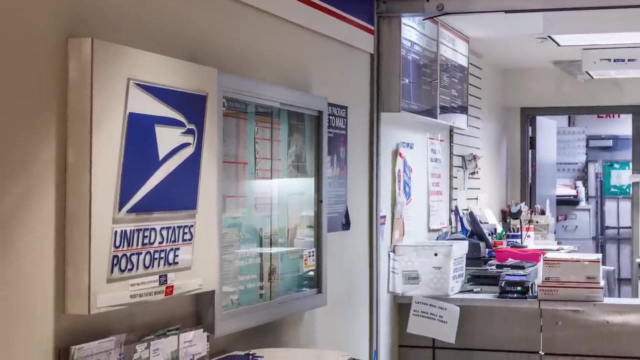 to our house and boy, i didn't realize how many- 600 plus- copies would be, and we literally filled an entire room just full of kickstarter stuff. also, have you ever tried to mail out over 600 packages? how do you do it? do you take it at the post office? do you just walk in and hand it? 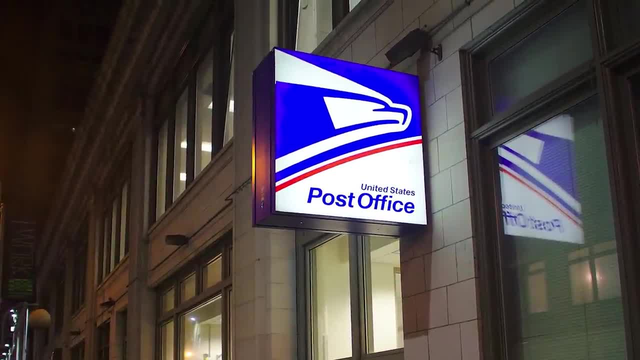 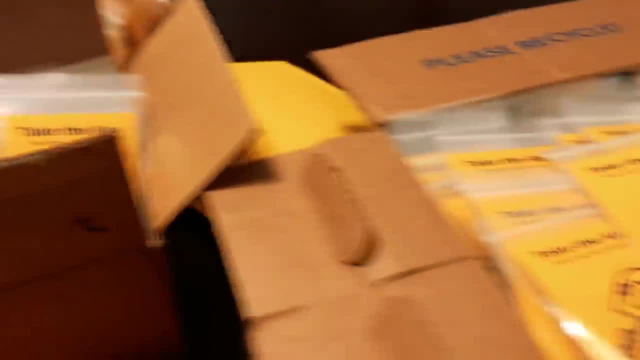 to them. there's so many little details that you don't even think about until you actually have to do it. so i get the fourth team together and we literally spent eight hours straight one day just packaging games and loading them up so we could go to the post office. 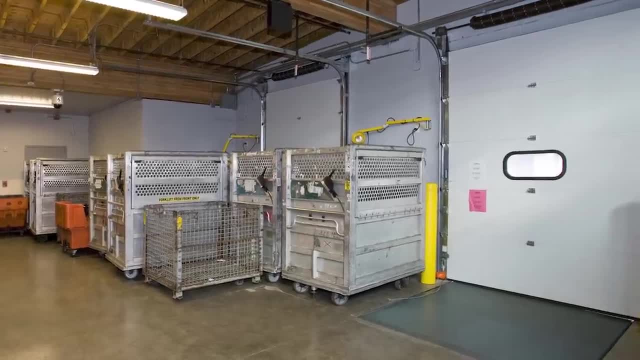 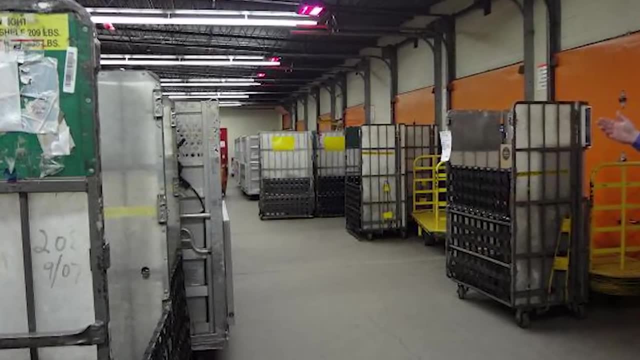 and then we had to go into a loading bay to drop off all these copies, which i've never done before, and it was a very surreal experience and i actually got a tour of the post office, which was sweet. so i guess what i'm trying to say by all this is a lot of times when you do a kickstarter. 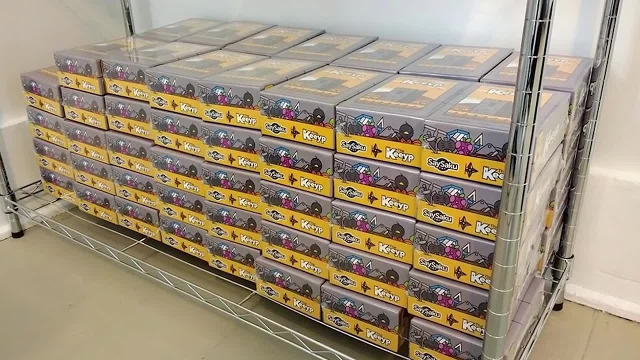 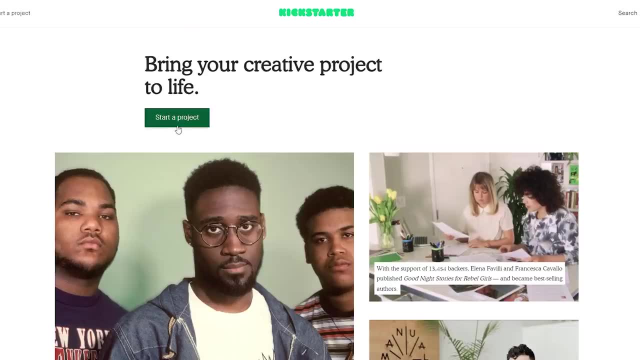 you don't realize how much work things are going to be. copies are going to be more expensive than you think they are. mailing is going to be more pricey or strange or harder to do than you think it's going to be. so if you're looking to do your own kickstarter, make sure to keep those things in. 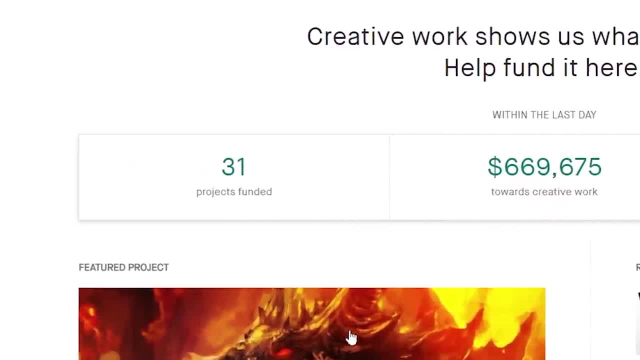 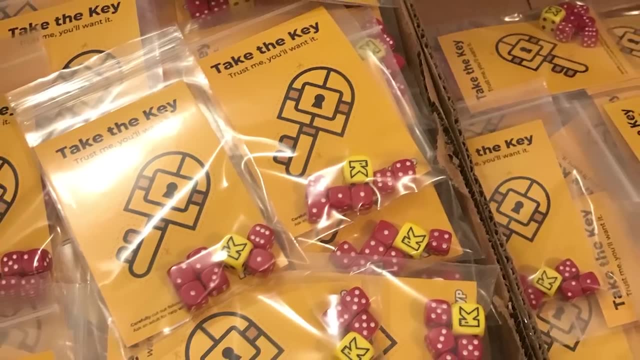 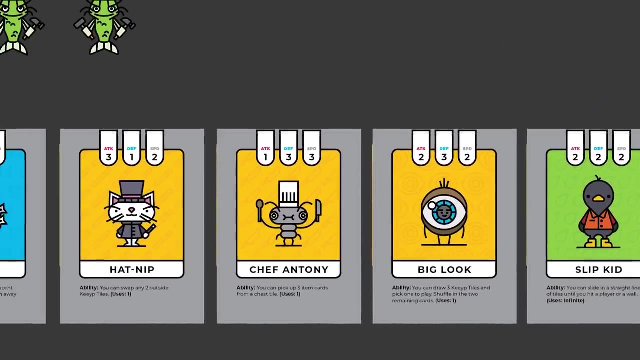 mind, as they can be scary when you have a lot of money and you're in the middle of it. now, if you and you didn't fill out the survey on kickstarter, please make sure to do it, otherwise we can't send you your copy, okay. so i kind of told you the story about the success we had with the keep. 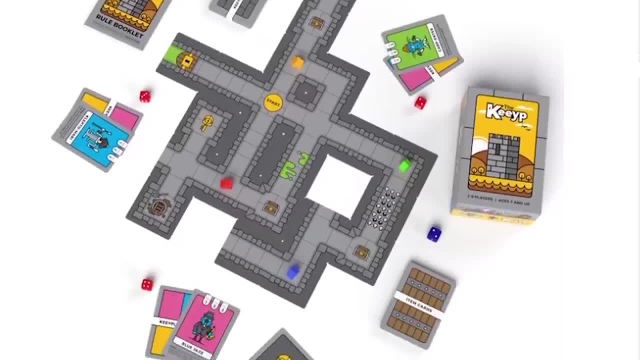 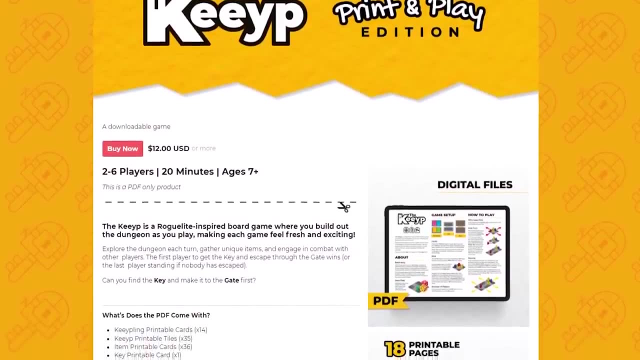 but what's next? what if you missed the kickstarter? what if you still want the game? well, we're doing everything we possibly can to make the game available. we made a print play version that you can buy on our itchio page. we also would love to release more physical copies, but our printer 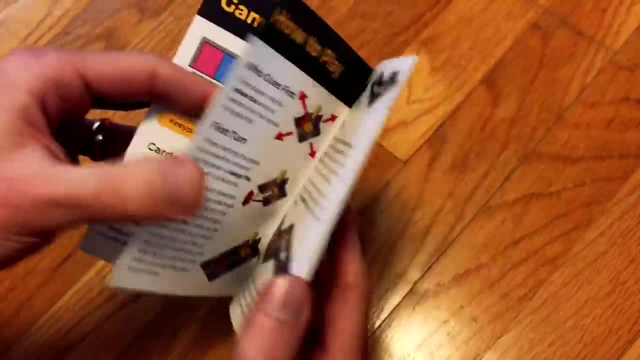 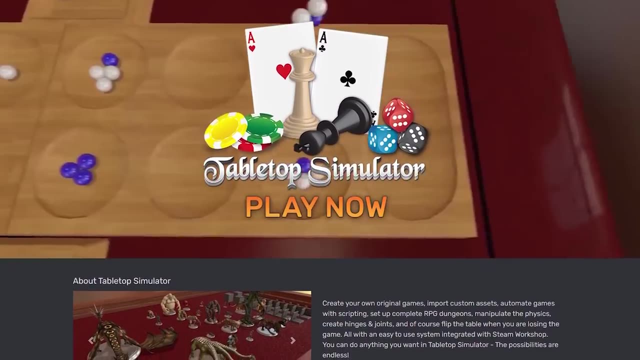 just isn't reliable and is really expensive. so if you know anyone who can print, well, let me know. and the third and final way we want to release the keep is through tabletop simulator. now here's the thing. we've actually been in contact with tabletop simulator and they actually want to. 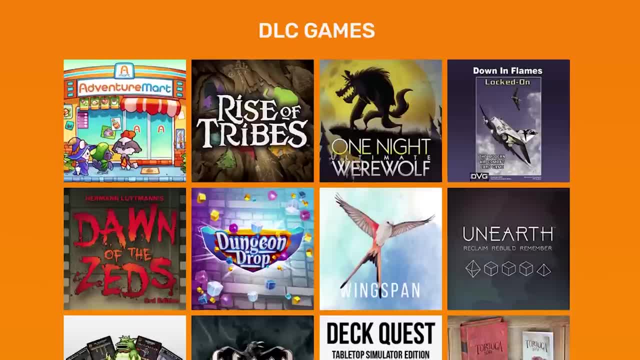 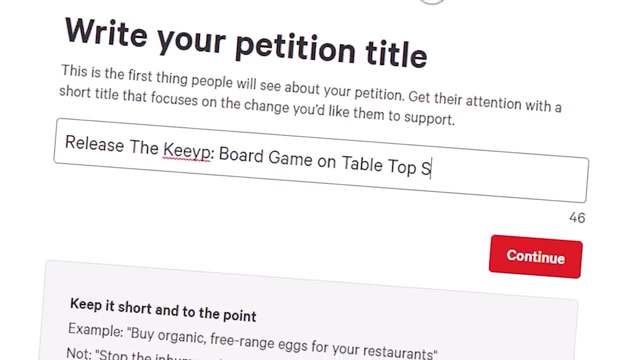 work with us, or at least that's what they said to us about six months ago, but we haven't heard from them since. so what i figured is that we should do another petition, a petition to get the keep on tabletop simulator. so if you'd like to see the keep on tabletop simulator as official dlc. 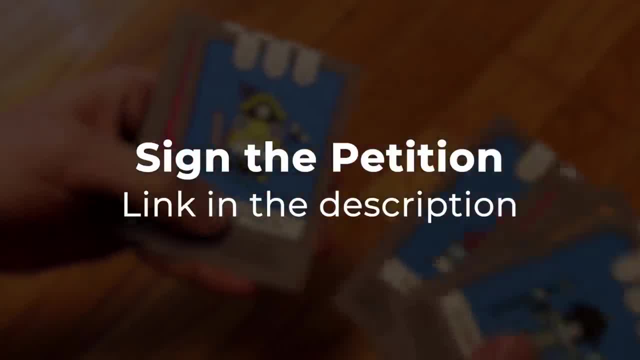 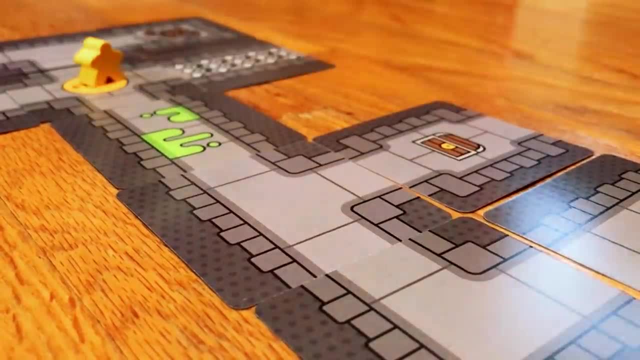 make sure to go in the description below and to sign the changeorg petition for it. it helps so much and it's completely free to do the keep has a bright future because of all of you guys and all of your support. i have six expansion ideas already in my 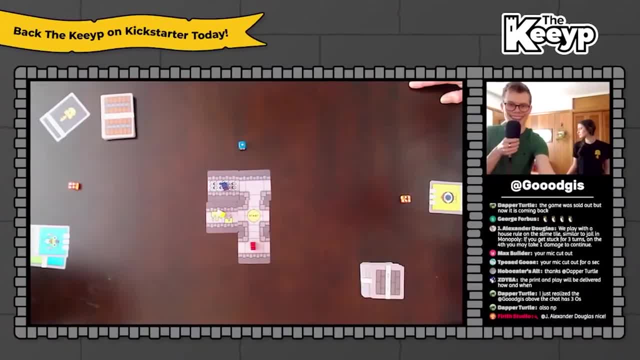 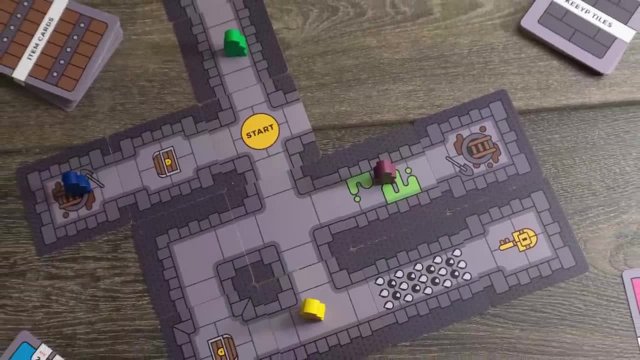 head, new keeplings, booster packs. maybe eventually we can even host tournaments with prizes. i have so many ideas, but i just want to thank everyone for making the keep possible. if it wasn't for you guys, i wouldn't be able to make this video today and the keep would still be sitting on my 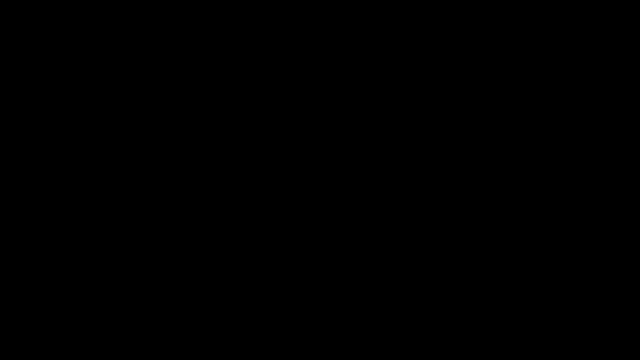 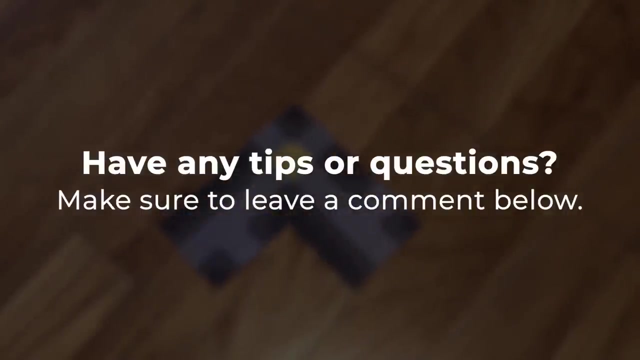 shelf, sad and lonely. so i want to ask you guys: have you played the keep on tabletop simulator? keep. do you like it? what's your thoughts on it? would you like to see it come back? what sort of expansions do you think would be cool? let me know in the comments down below. i love reading your. 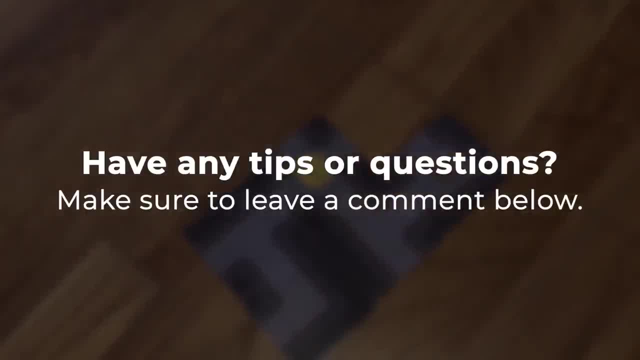 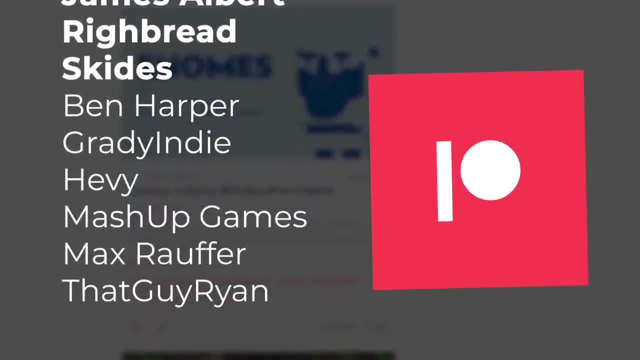 guys's comments. i reply to every single one of them, so thank you so much. also, just a huge shout out to rye bread, james albert, heath sergeant and skydes and the rest of the fantastic patreon supporters that really make these videos possible. you guys are fantastic and i appreciate you so.